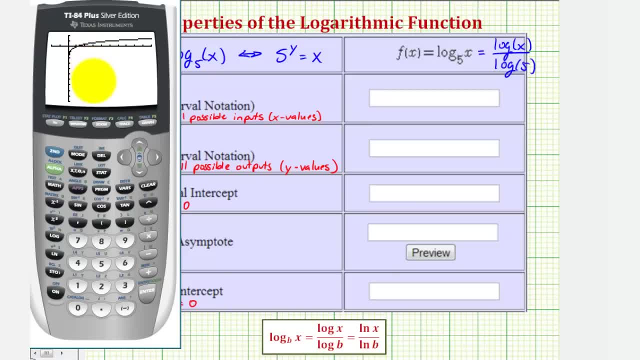 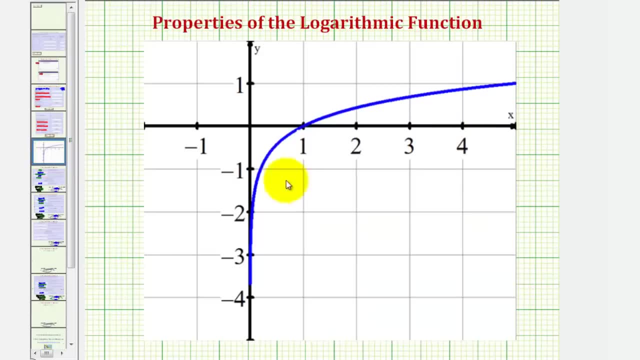 which we will use to answer some of the questions. But I did reproduce this graph on some different software so we can better analyze the graph. So we'll actually be using this graph here to analyze the log function. The first question asks for the domain. 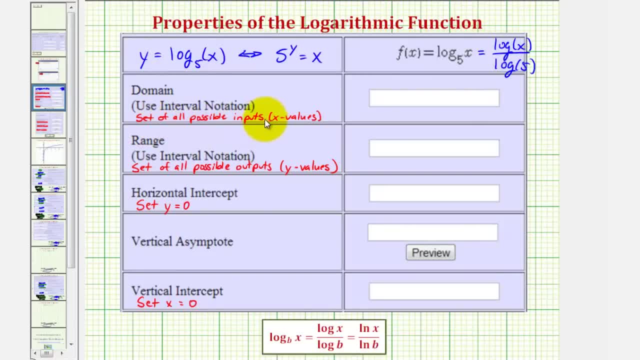 of the logarithmic function, which is the set of all possible inputs, or all possible x values. To do this analytically, I think it's helpful to look at the exponential equation. here We're thinking about what values we can get for x. 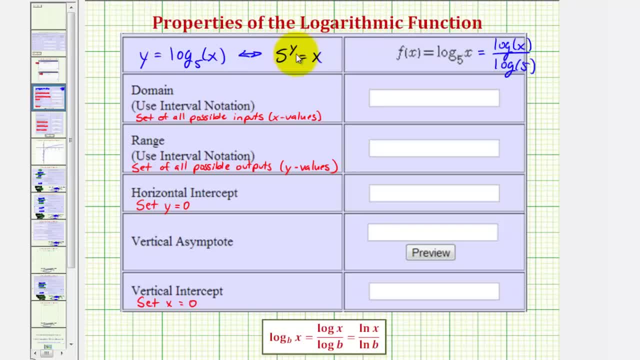 if x is equal to five raised to the power of y. Whatever power we raise five to x is never going to be negative. It's also never going to equal zero And therefore the domain would be: x is greater than zero or the open interval from zero to infinity. 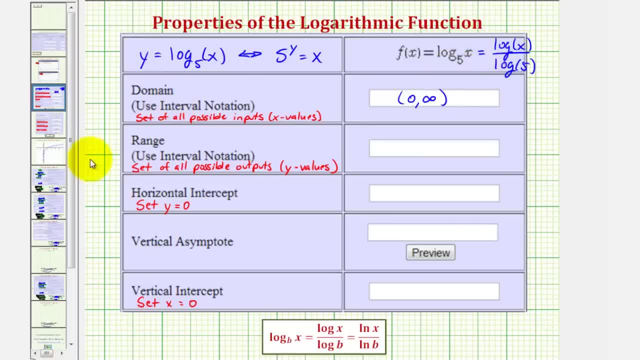 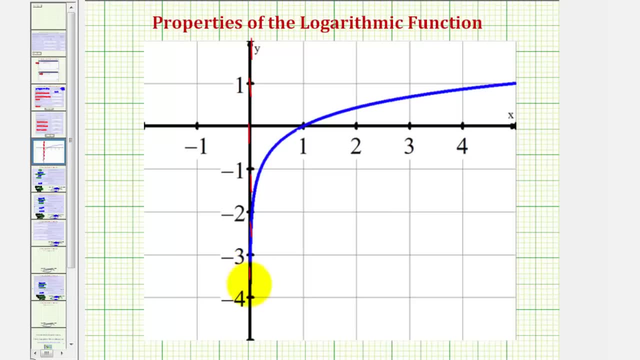 using interval notation. If we look at the graph of our function, notice how it never equals zero because we have a vertical asymptote here. Notice the x values are only to the right. of x equals zero. verifying the domain is the open interval from zero to infinity. 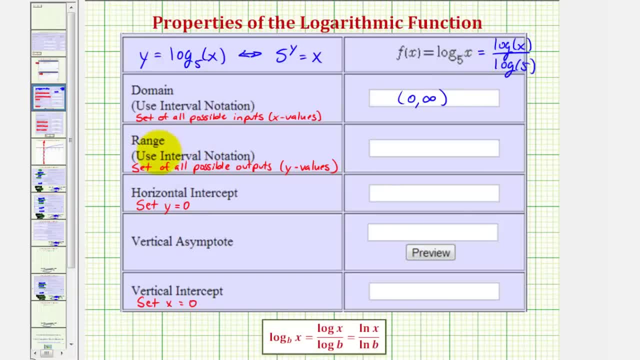 Next, we're asked about the range of the log function. Again, looking at the exponential form, notice how we can raise five to any real number and therefore the range would be all real numbers or the open interval from negative infinity to positive infinity. 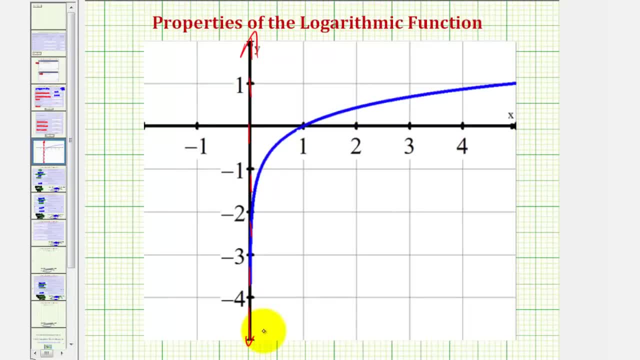 Going back to the graph, notice how the graph goes down forever and even though it is moving right very quickly, it's also moving up forever With no breaks. verifying our range is all real numbers or the interval from negative infinity to positive infinity. 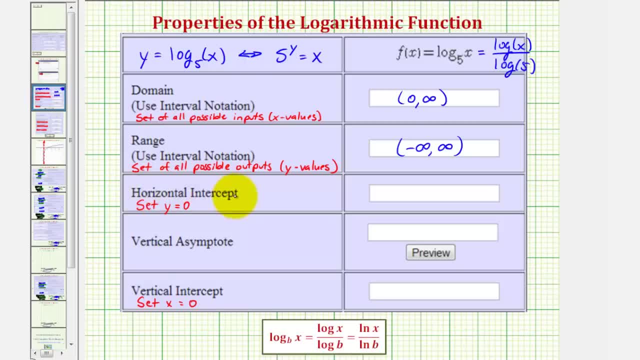 And now to find the horizontal intercept, which is the same as the x intercept, we set f of x or y equal to zero and solve for x. To do this we'll use the exponential form. Notice how, if we set y equal to zero, 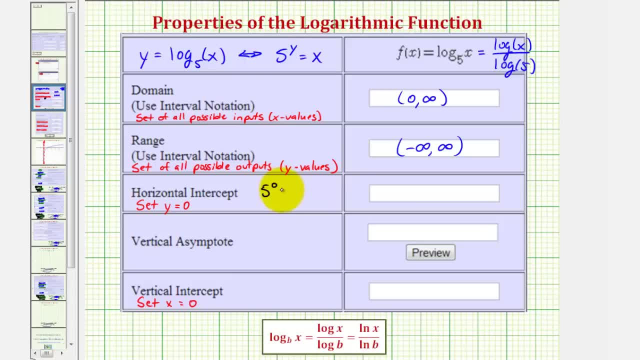 we would have the equation: five to the zero equals x. so x equals five to the zero, which is equal to one. So if the x intercept or horizontal intercept is one, we're at the point one comma zero. We can easily verify this on the graph. 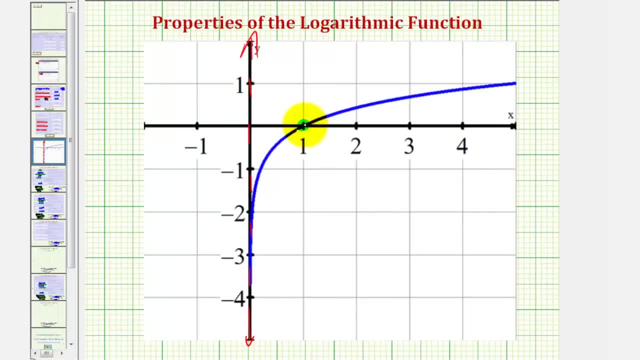 Here's the horizontal intercept, which is the point one comma zero. Next we're asked to find the vertical asymptote and we briefly discussed that. Notice how, as x approaches zero from the right side, the function values decrease without bound and approach negative infinity. 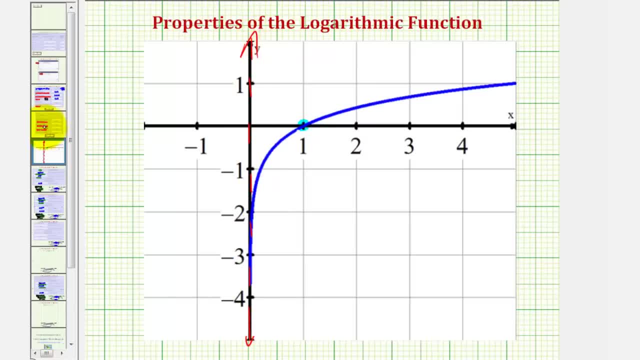 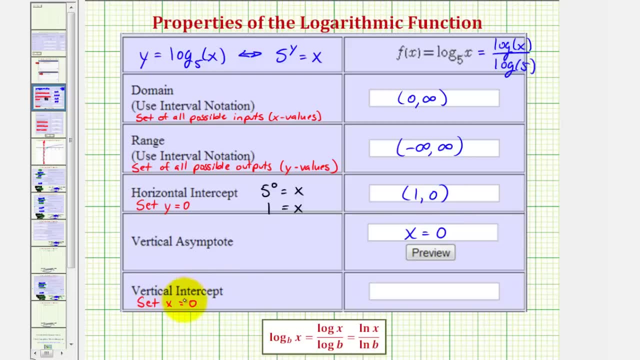 and therefore we have a vertical asymptote at x equals zero. Next we're asked to find the vertical intercept, which would be the same as the y intercept. so we set x equal to zero and solve for y, So, again using the exponential form. 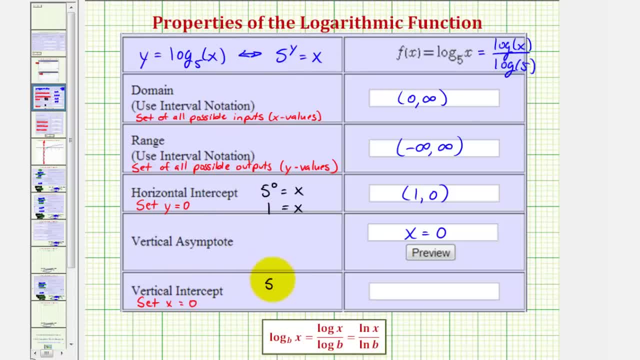 if we set x equal to zero, this would give us the equation: five to the power of y equals zero, And we discussed earlier, we can't raise five to a power to the value of zero. It's always going to be positive. 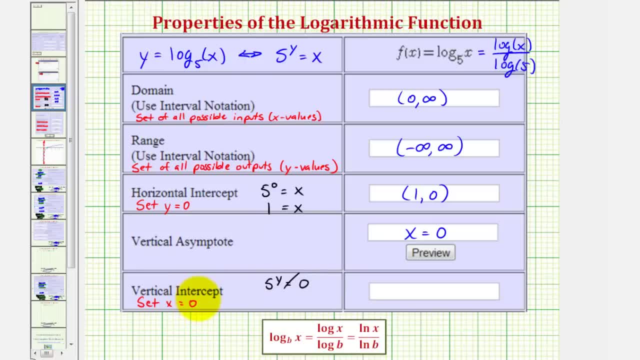 and therefore this does not have a solution. which means we do not have a vertical intercept or we do not have a y intercept, So for the homework we'll type in dne, for does not exist. Now. we're not done here. 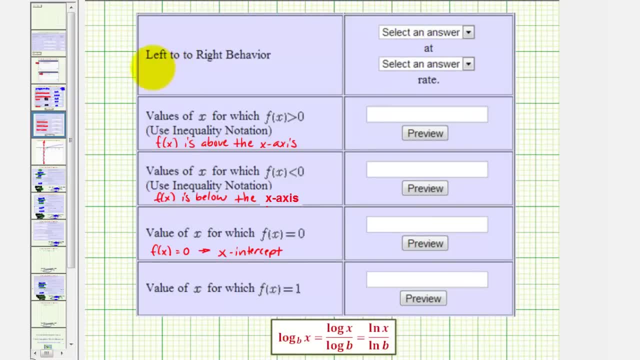 we still have more questions And notice there's a typo here that should say what is the left to right behavior, describing it as increasing, decreasing or constant. So, going back to the graph, notice, as x increases, the function values also increase. 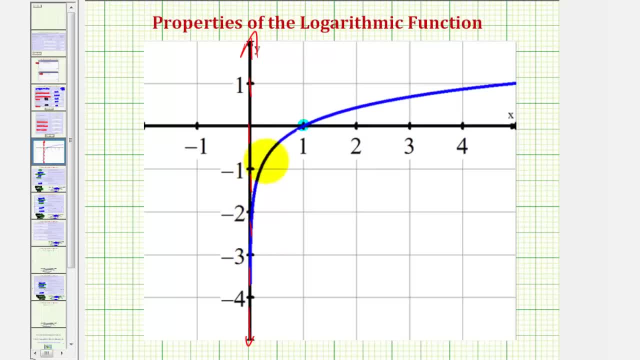 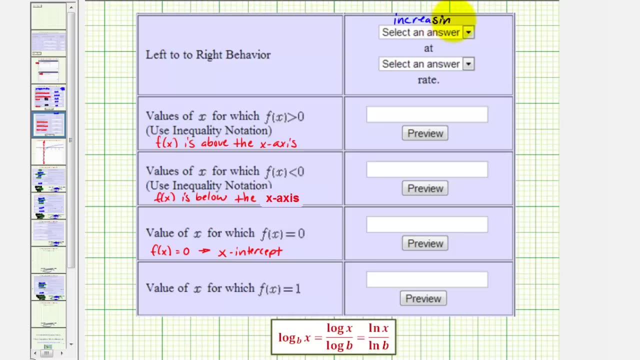 so the function is always increasing, but notice, as x increases, it does not increase as fast and therefore we can say: this function is increasing, but it's increasing at a decreasing rate. So again, this answer here is: it's increasing. 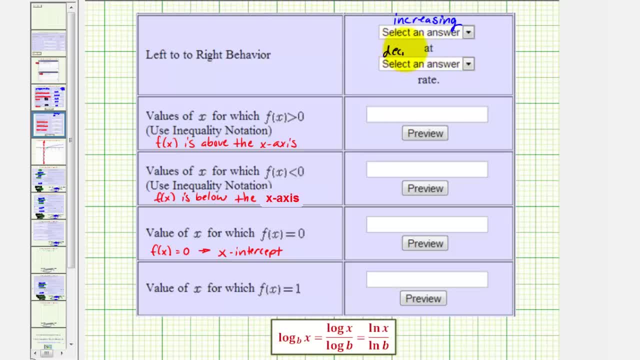 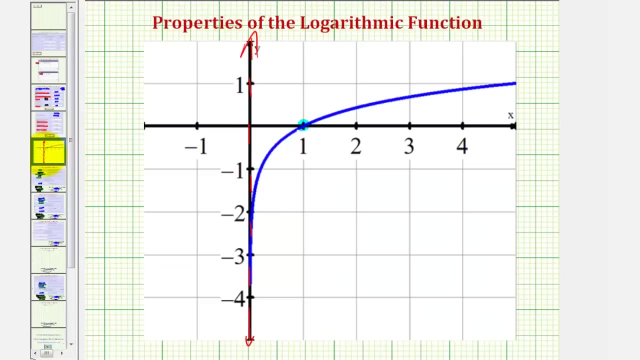 but it's increasing at a decreasing rate. Next, we're asked to determine the values when the function is greater than zero, which would be when the function is above the x axis. So, looking at our graph, notice how the function values, or y values. 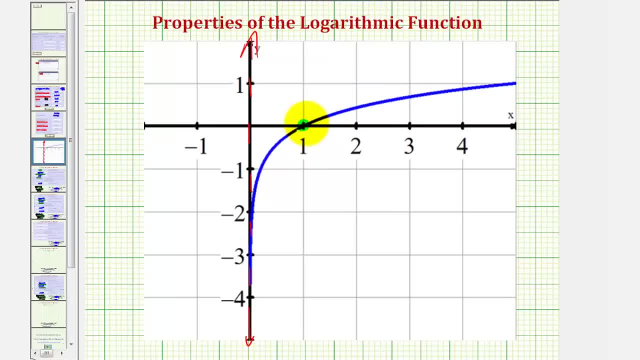 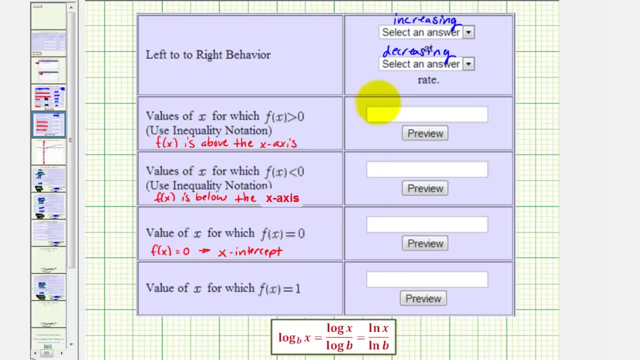 are greater than zero or positive above the x axis, and therefore we can say the function is positive when x is greater than one. Notice how it does ask us to use inequality notation, not interval notation, So we'll type in: